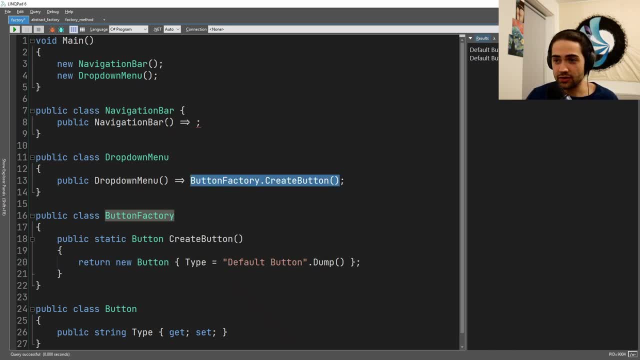 And create a button. Now, instead of changing it in a thousand places, we only need to change it in one place. Okay, we're on it and we got the red button. So if you're ever looking for like a symptom, when do I need to use a factory pattern, be it whatever. whichever one you want to use of the ones that we're going to go over, It is generally: am I creating something in two places identically? If so, 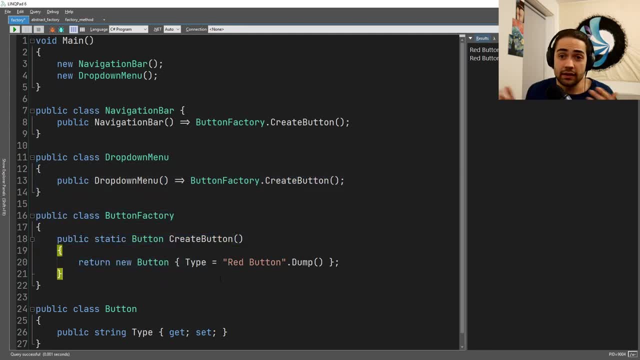 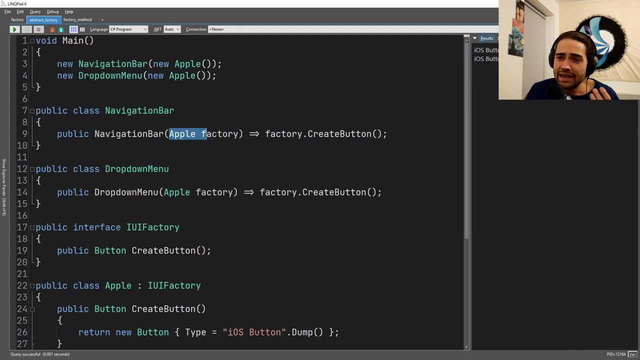 bring it in one place. All right. In this case the button is internal. We don't need anything from outside controlling how it looks like. Just keep it in house, Doesn't matter. Usually this could be like a helper method sort of thing in your application. Okay, The simplest thing possible. All right, Let's move to the abstract factory. Okay, Same scenario: Navigation bar drop down menu. We are rendering these for specifically for an Apple phone. All right. 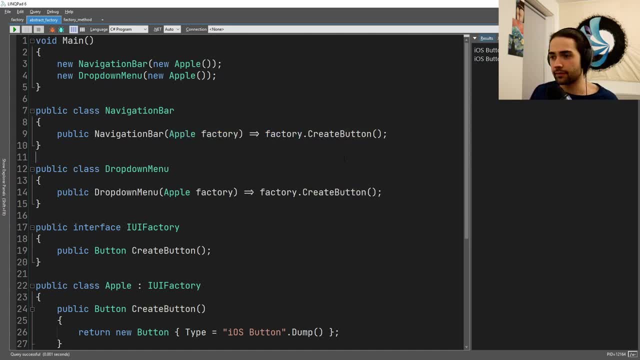 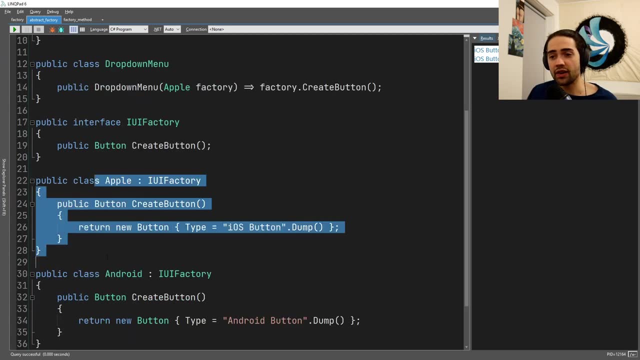 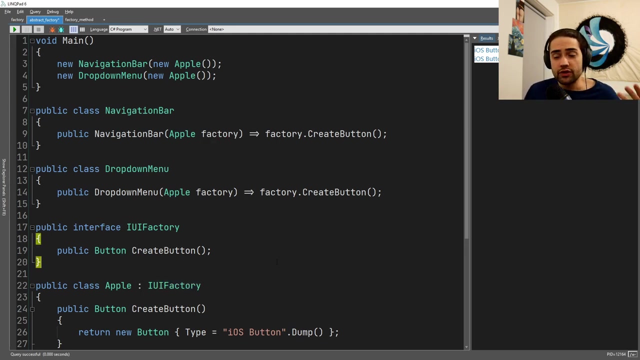 All right, So we take the factory and we create a button. Okay, So for both of these, on the navigation bar in the drop down menu, we have an iOS button rendered. Now I do have my Apple class already inheriting from UI factory, And this is just because I've set up the example like that. But imagine we didn't have something like that. Okay, And this was just a button factory. Okay, So what you want to do in order to allow something externally to control how your application looks like? 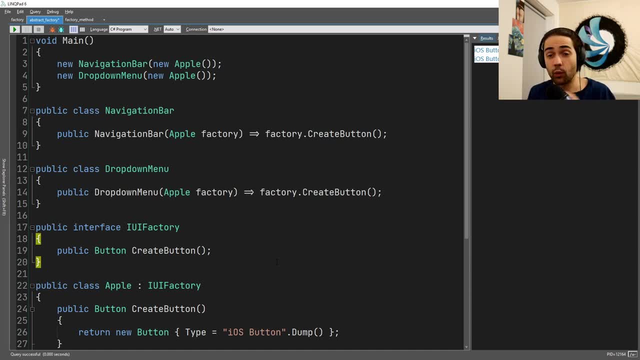 For example, if a very popular one is dark mode and light mode, right, It's just two different color schemes. If we could basically have a theme interface and then light mode and dark mode, we just basically switch between the two implementations and all elements change colors. All right, Same principle here. Here we're only confined to the Apple example. We go ahead and give it an interface. Now we're no longer. 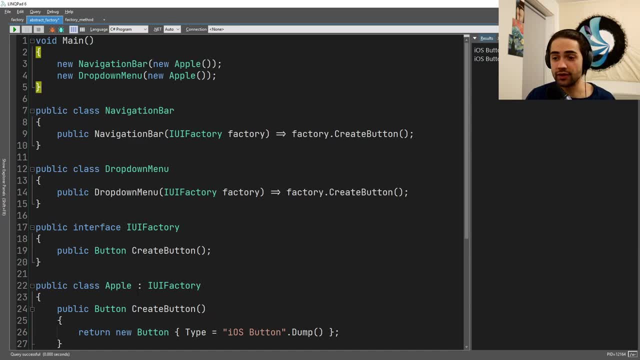 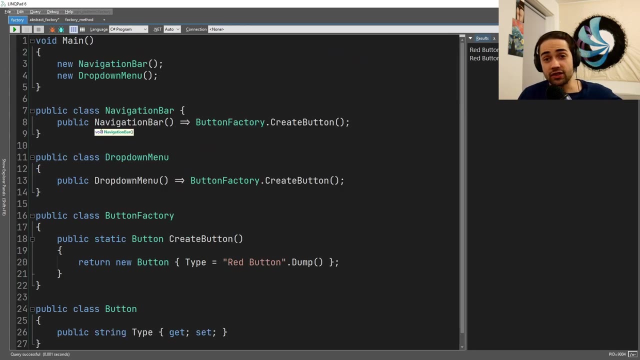 confined to just the Apple example, although we can still use it. We can then just go ahead, grab the Android implementation and put it in there, Right. So this, the abstract factory, is again. we sort of took everything that we could, We segregated it Right, But because in the factory example it was only used internally and we don't need something externally to control how our application works, We keep it in house. Now, this is where we need to offset or abstract our 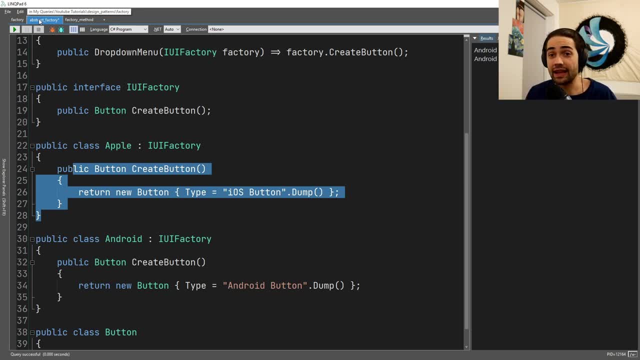 how we want to create these things. This concept is also known as dependency inversion. This is where we define what we need, but the thing that is going to do the actual creation is the thing that is supplied. Okay, So we say that we have a theme, This is the template for the theme, and the actual implementations for the themes are all different. Right, And I can have different color sets and they can just be like sort of thrown into onto your color palette with different colors in there. 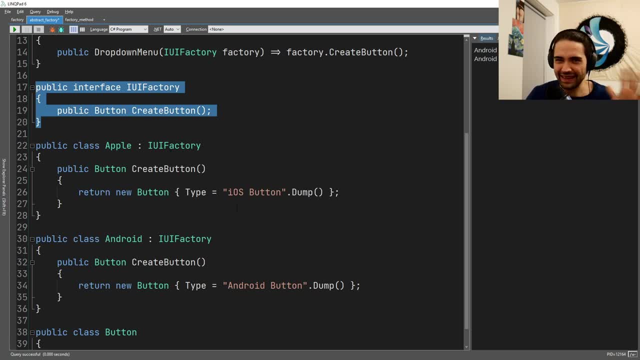 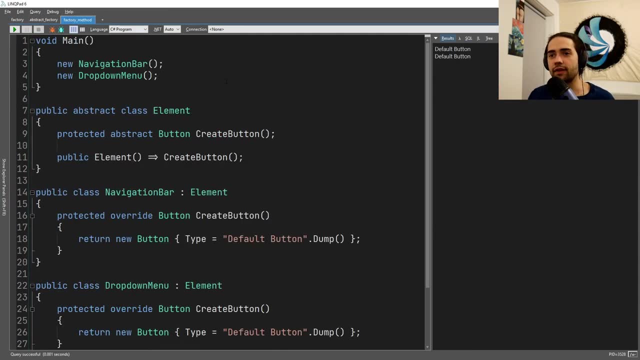 And pick from them. Okay, So that kind of thing is going on here. We're injecting, Think about injection. Think about composition, dependency, inversion. Okay, Let's take a look at the factory method. Now, this one was a little bit hard for me to grasp at first, because I've never actually used this consciously. All right, We will come back and look at the abstract factory and see how factory methods are actually used there, Although, again, as I said in the beginning, it doesn't matter so much if you exactly 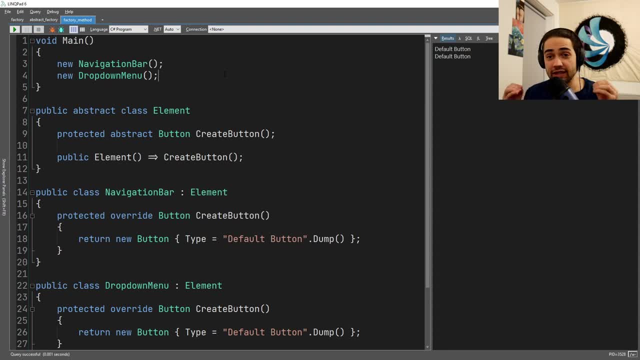 know which factory pattern you're using. Understand, if you're just getting rid of duplication and giving more structure to your code by making sure the way that you create objects is in an organized place, you're kind of already doing it. So in this example we have a navigation bar, We have a drop down menu. We run the both and we both. we get default button from both of them. Now we have an abstract element where we have the factory method: create button Right. 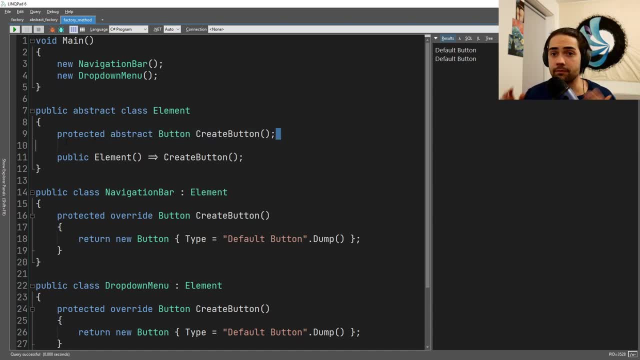 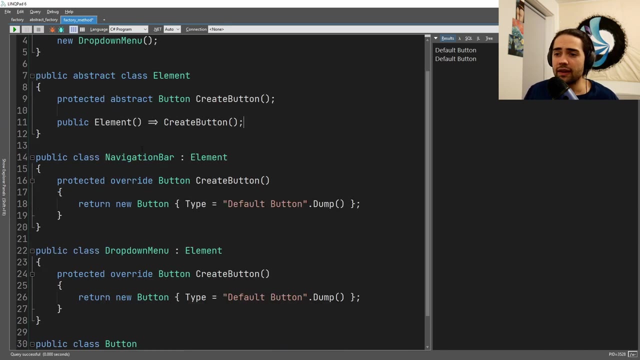 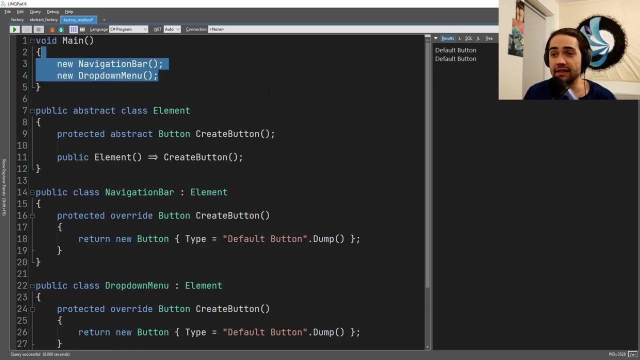 So it's just an abstract class that we can implement. Okay, So this is going to be quite important. We have an abstract thing that we can implement, just a method. This means we can have multiples of them, Each individual one of these is a factory method. Okay, We then have the navigation bar and we have the drop down menu. These are our building blocks with which we can organize this thing. So what can we do further to sort of enhance the 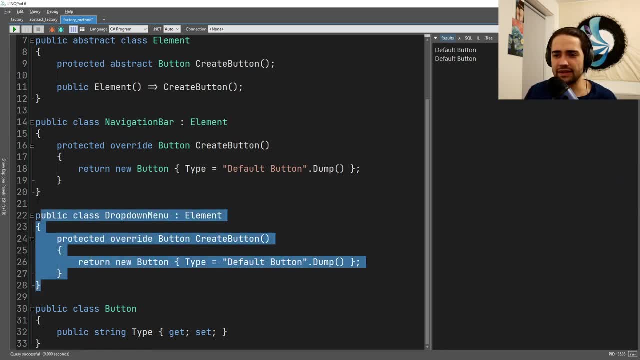 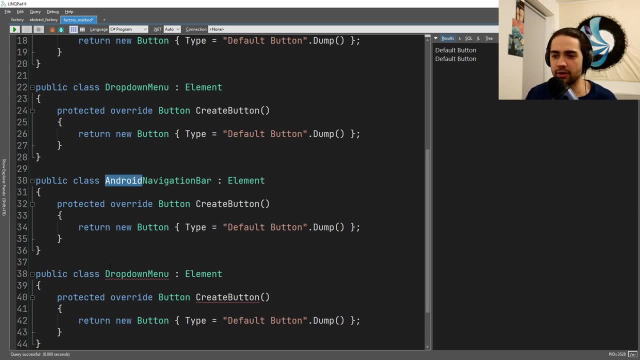 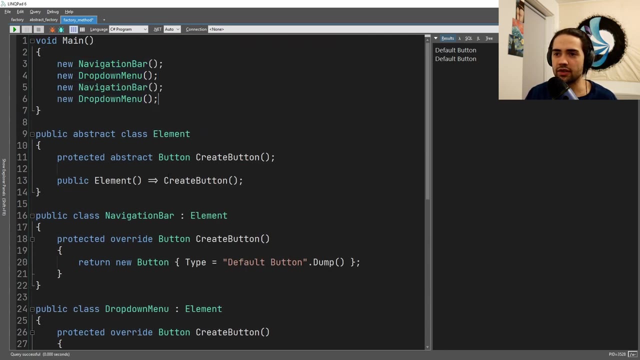 or basically, how do we use our building blocks in this case? Well, here what we can do is we can basically do something like this: Let's say, Android navigation bar, Android drop down, line up, and then have Android in these two places, And now we have essentially four objects to pick from. And there we go. So think about it: We have added tools to our arsenal And instead, 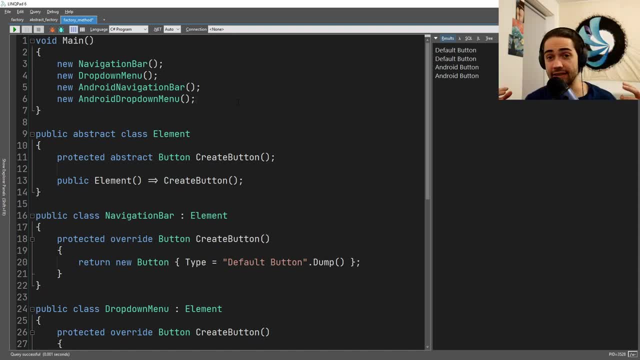 of injection. we are now using inheritance to enforce the structure of having a button created for these elements. Now, to kind of break down the difference between inheritance and injection, composition and still inheritance- right, these two areas, and when do you want to use which one? composition is ultimately flexibility and inheritance is structure. you need to balance these two inheritance. 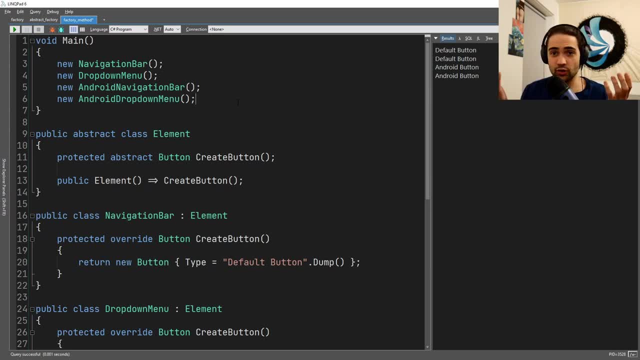 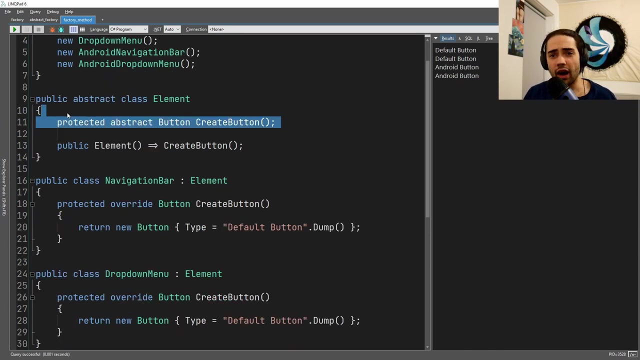 order to get software. If you go full composition, you just have a set of random things flying around which you have to put together. you basically end up having infinite utility If you have. if you go full structure, you're rigid, you can't change, So generally you want to balance two things together. Now to come back to the abstract factory example, where we are indeed using a factory method. in the abstract factory it is: 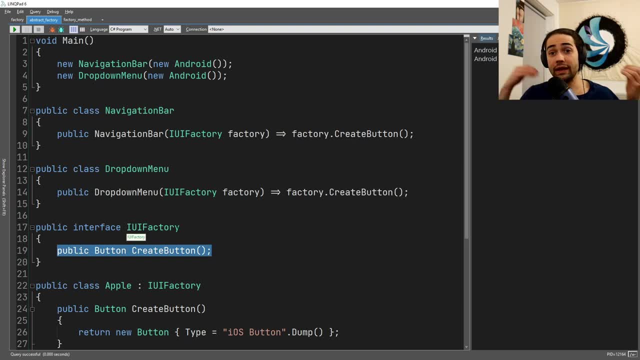 So here on our interface and then goes somewhere else, you're CRISP class. we have a factory method that we want to overwrite right and that's essentially a factor. factory method is a factory method. if we have multiple factory methods on an abstract factory, that is still a factory method. a simple factory that just creates something that you just need in your code base as a utility in just use that Right. So hopefully you that it's still a factory method. I think this concept a little better and